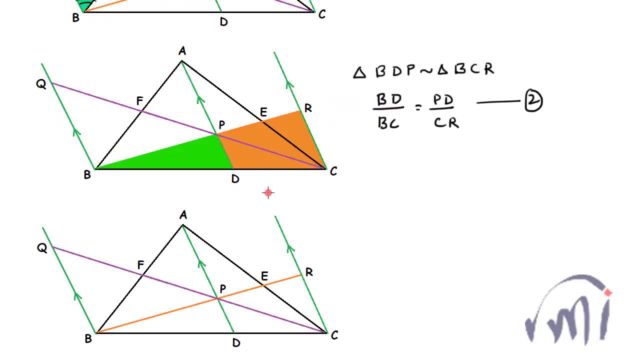 So here we got an equation in terms of BD and of we try to find the equation in terms of DC. so here we will compare this triangle that is triangle CDP and this triangle that is triangle CBQ. Both of them are similar triangles. that means ratio of DC to BC will be equal to this value here. 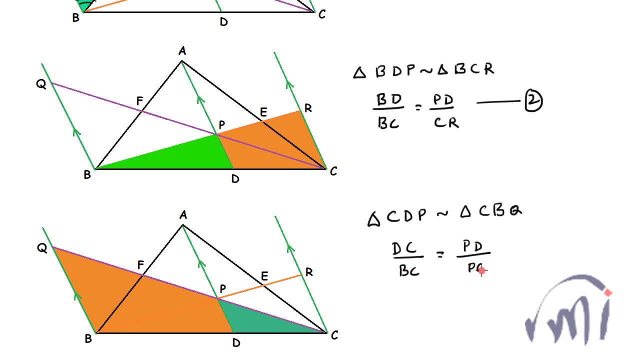 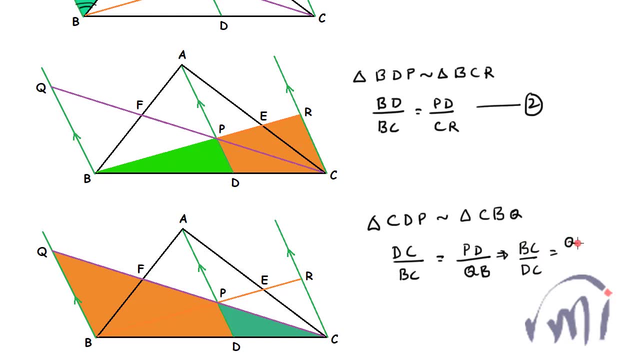 So we will write here Diggle of BC and this like this triangle, CDP, and this like this triangle, CBQ. So this is a counter from this where the radius D is 31.. to PD divided by QB, or you can write it as PC divided by DC, is equal to QB. 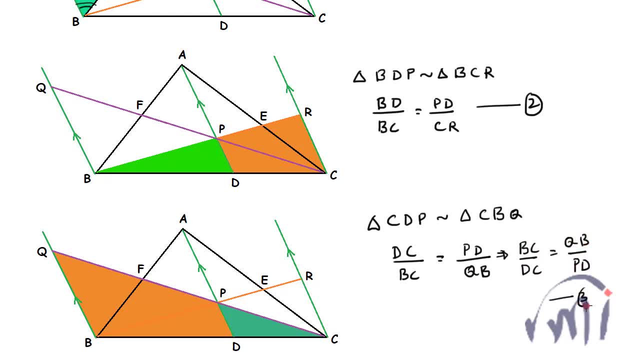 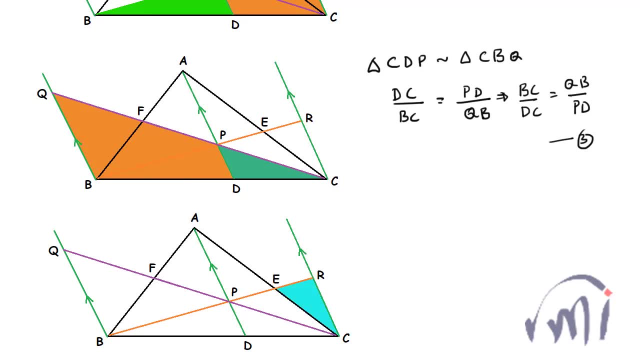 divided by PD. Let me call this as equation number 3, and now we want an equation in terms of CE and EA. So I'll compare this triangle and this triangle Here. also, this angle is equal to this angle. vertically opposite angles and this angle is equal to this angle. alternate angles between two parallel. 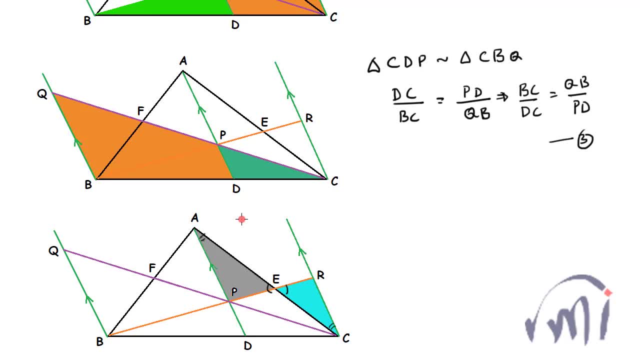 lines. So remaining angle will also be equal and these two triangles will be similar. So we can say triangle ECR is similar to triangle EAP. or you can say EC divided by AE. The ratio of these two sides will be equal to CR divided by. 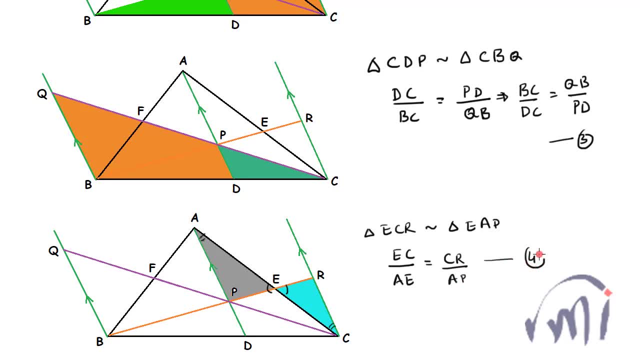 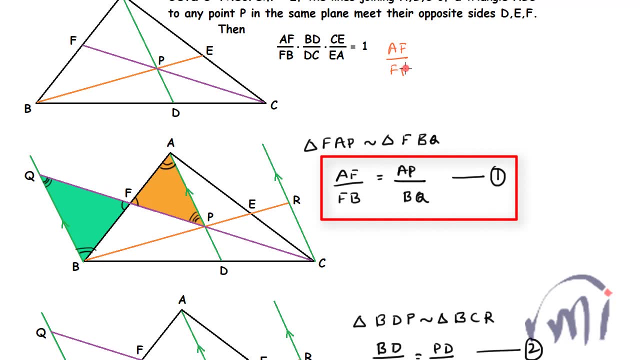 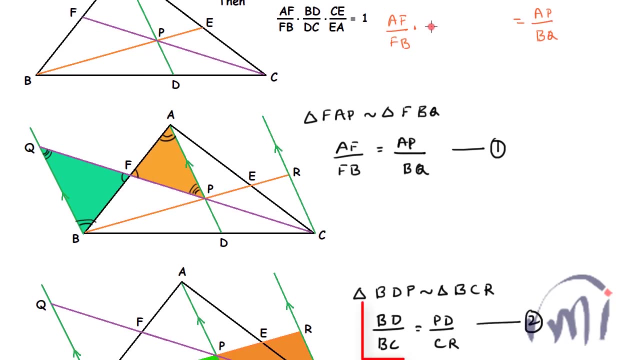 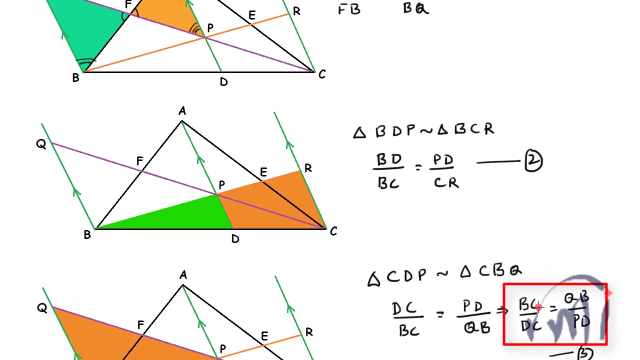 AP. Let me call this as equation number 4. and now let us multiply all these four equations. so I'll get AF divided by FB, which was equal to AP. divided by BQ, multiplied by the second equation, I'll get BD divided by BC, this will be equal to- I have to multiply the right hand side to the right hand side- PD divided by CR, and then I have to multiply the third equation, which is equal to BC. 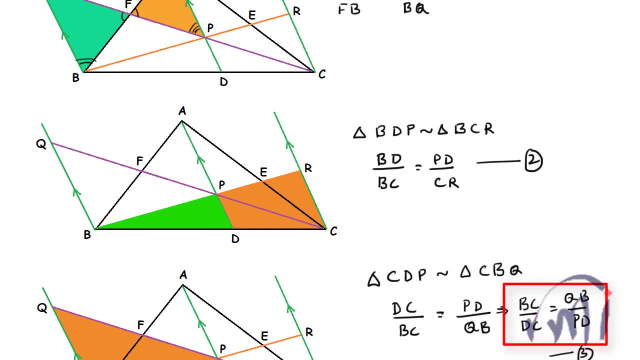 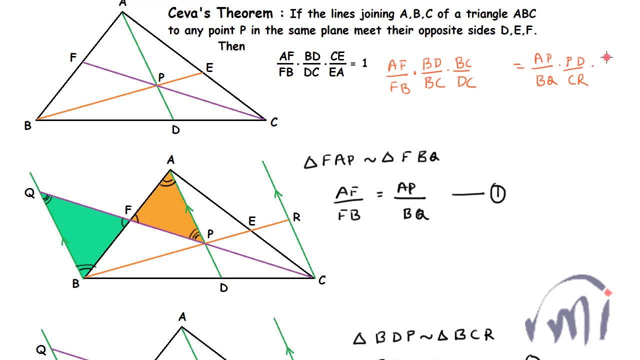 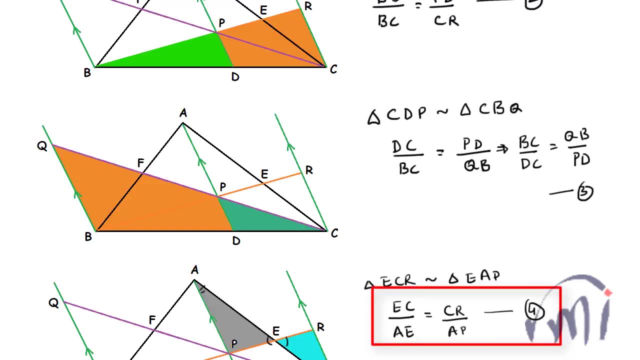 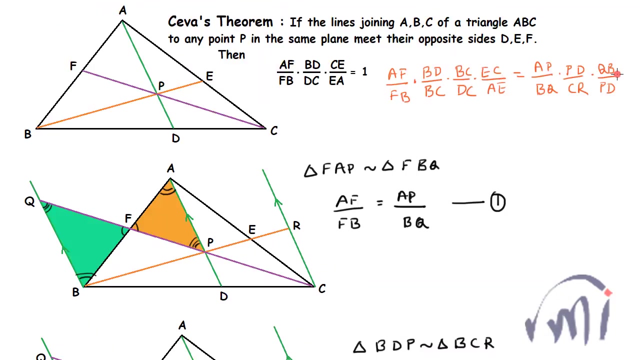 divided by DC is equal to QB divided by PD. so multiplied by BC divided by DC, and this was equal to QB divided by PD. and the fourth equation was: EC divided by AE is equal to CR divided by AP. EC divided by AE is equal to CR divided by AP. so here,